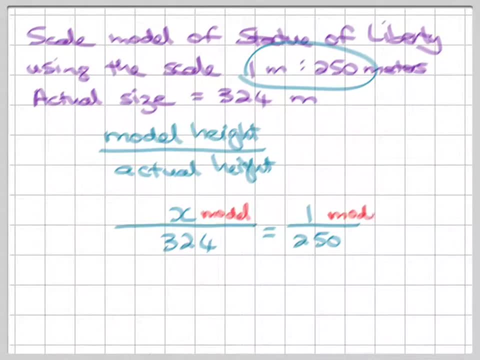 and that's also the model. so you keep the correct units on both sides. This is actual and that's also actual. Okay, now we're going to cross multiply, so we're going to go like that. that will be 250. x is equal to 324. now we divide by 250 on both sides to isolate our x. x is equal to. we're going to 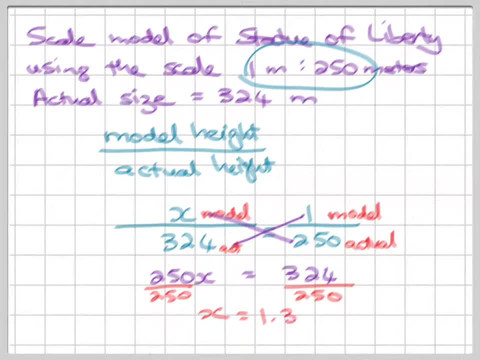 round it, I think it's 1.3, 1.3 meters, so our model is going to be 1.3 meters. it comes to 1.298 or something. I've rounded it up So you can see how easy it is, and I want you to bend. 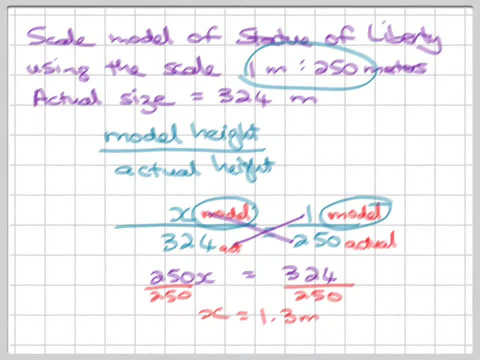 mind it's always the same units on the other side of your proportion- actual for actual, model for model- and then you cross, multiply and you would really have no problem finding the right answer. if you stick to those rules, I'll see you in tomorrow's lecture. 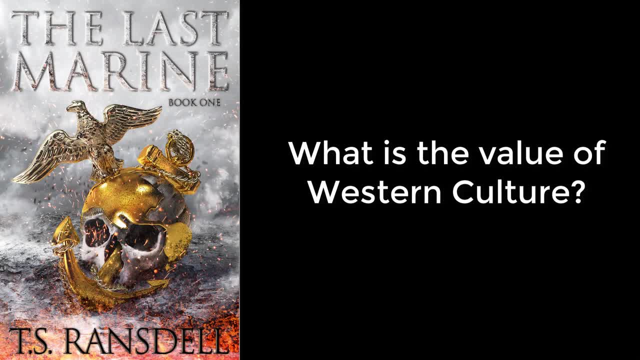 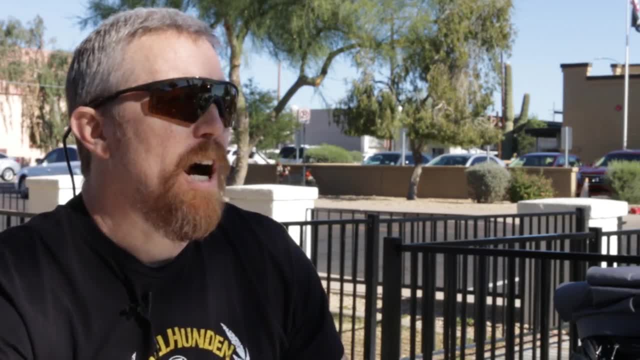 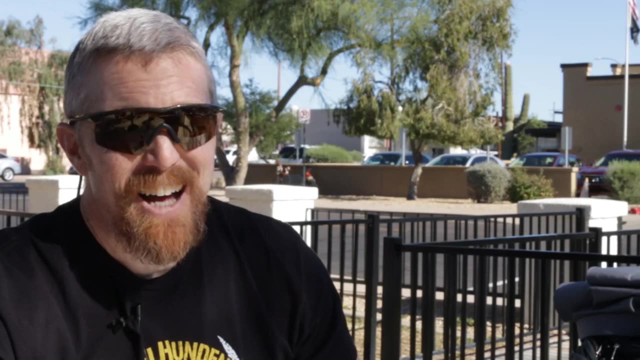 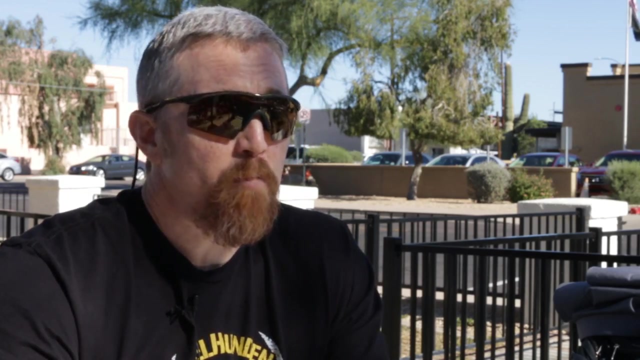 Culture determines how we will live as a people and whether or not we will survive. I think the main value of Western culture, of American culture, it's a culture that values individuals. It's a culture that values individual freedom, individual life, the freedom to pursue your 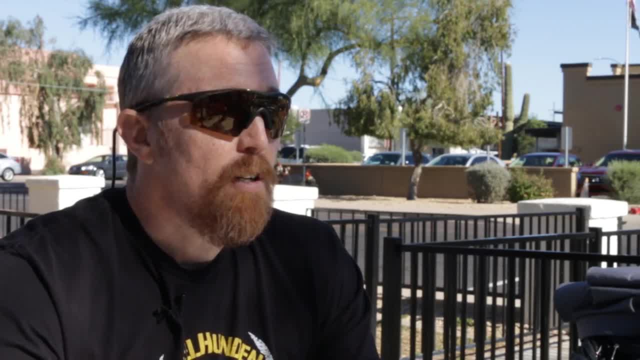 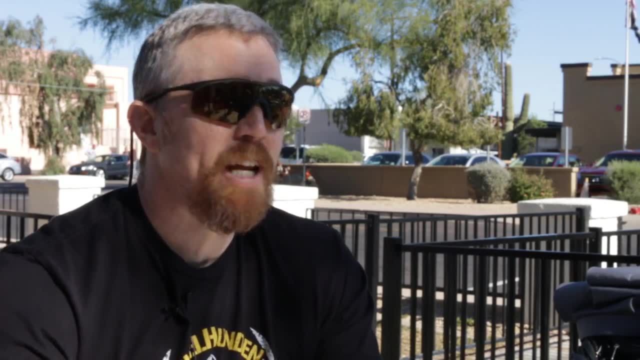 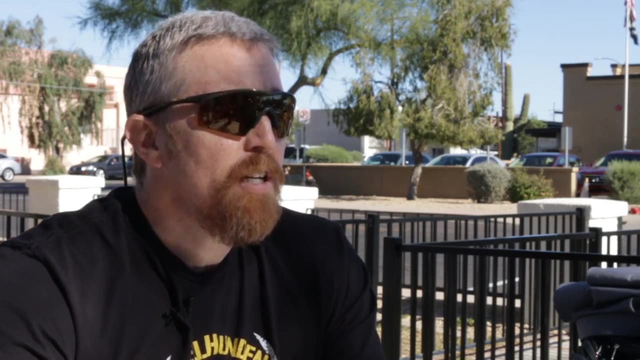 happiness to go out and do what you want to do. A lot of people don't have that. Cuba, for example- it's been the headlines with Castro dying lately. These people did not have that freedom. I remember growing up in the 70s how many Russians were always trying. 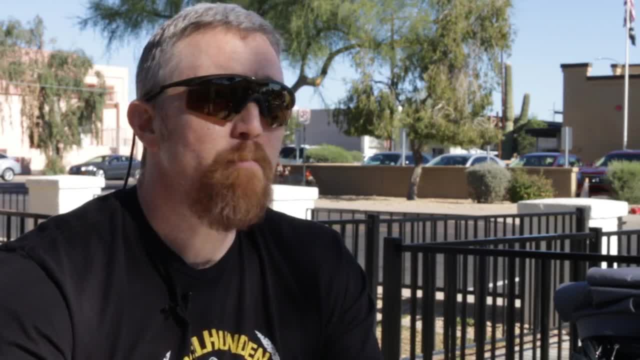 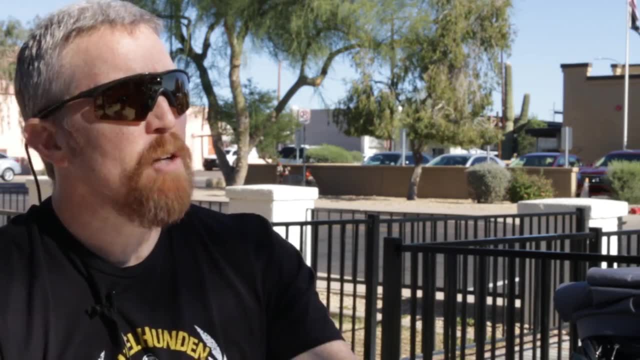 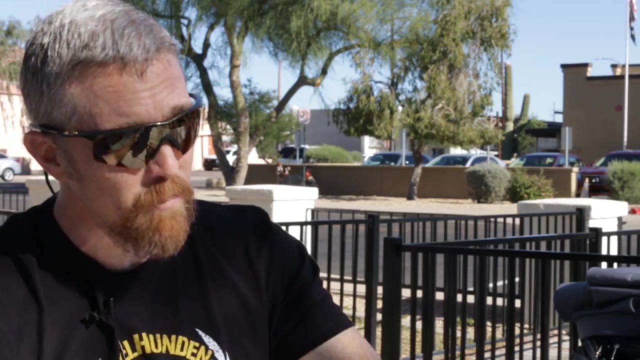 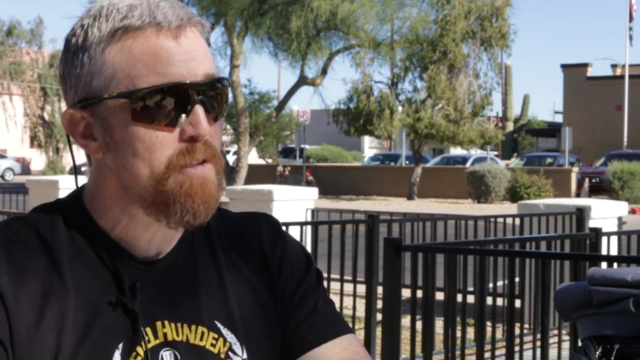 to escape out of Russia at the threat of family members being imprisoned or executed just because they wanted to be free. So there's value. Culture determines what we value, and if you're in a culture that values freedom and individualism, you're going to be better off than if you're in a culture that values collectivism and